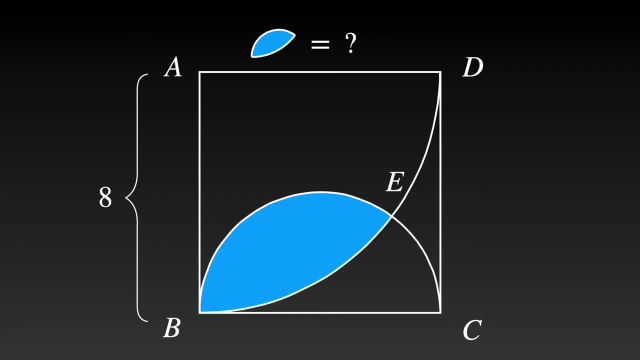 If you want to have a try, please pause the video. If you are ready now let's get started. Get the center of the semicircle O along line segment BC. Construct line segments AE, OE and BE Shade the shapes in red and green as shown. 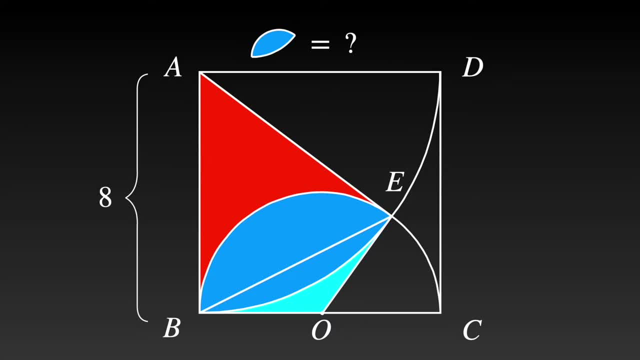 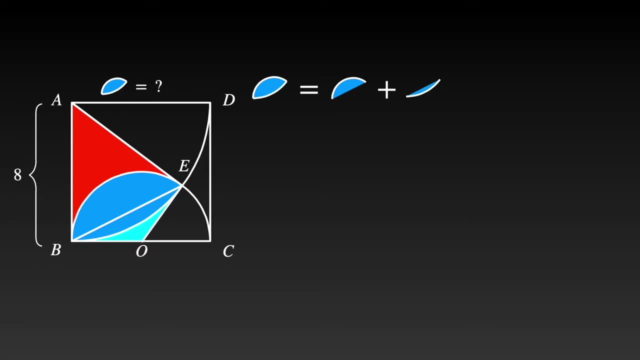 Then let's figure out how to get the area of the blue shape. The blue shape can be divided into two parts. The bigger part of the blue shape is equal to a sector subtracts the green triangle, And the smaller one is equal to another sector subtracts the red triangle. 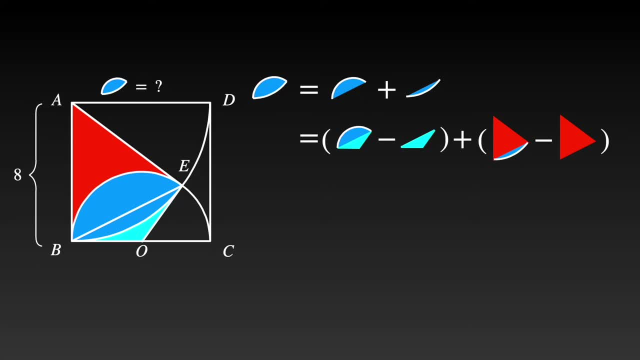 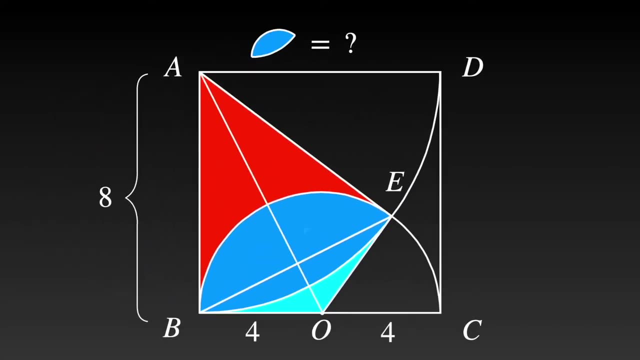 So the question is how to get the areas of the sectors and triangles Construct. AO and AB is equal to AE because they are the radii of the quarter circle And similarly, OB is equal to OE because they are the radii of the semicircle. 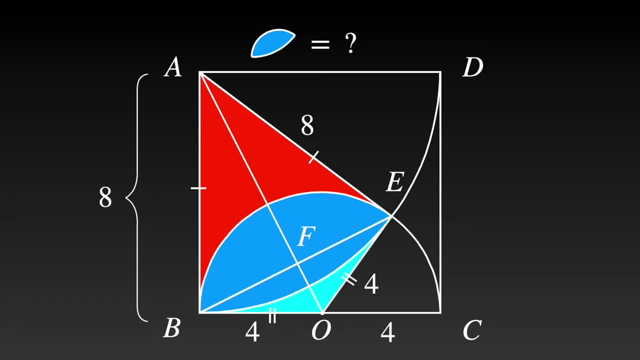 So the triangles AOB and AOE are congruent, which means the angle OAB is equal to angle OAE. Label the angles as alpha Angle. ABO is equal to angle AEO is equal to 90 degrees. So in the red triangle AOB tangent alpha is equal to OB over AB, which is equal to one half. 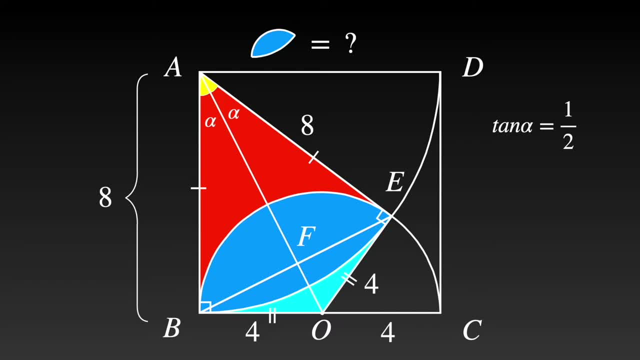 Triangles ABF and AEF are congruent, so angle AFB is equal to angle AFE, which means AF is perpendicular to BE, So angle OBF is equal to angle OEF is equal to alpha. That's what we will use in the next step. 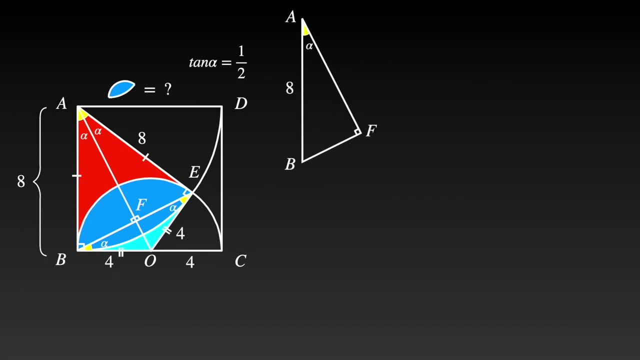 In the red triangle ABF, the hypotenuse AB is equal to 8,, which is the side length of the square. BF over AF is equal to tangent alpha, which is equal to one half And equal to persegarine theorem. square root of AF squared plus BF squared is equal to 8 squared. 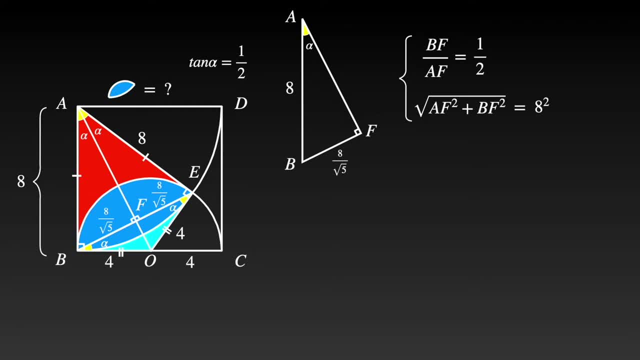 So, of the equations we got, BF is equal to 8 over square root of 5, and AF is equal to 16 over square root of 5.. In the sector ABE, AB is equal to 8, as mentioned above, and angle BAE is equal to 2 times alpha. 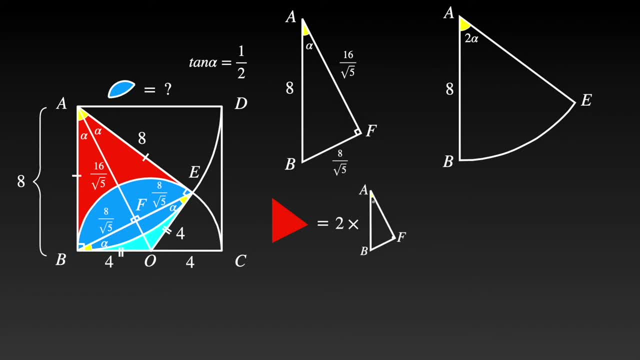 So the area of the right triangle is equal to 2 times the area of the right triangle, ABF, Which is equal to 2 times one half times AF times BF. Substitute the side lengths of AF and BF We got the result is equal to 128 over 5.. 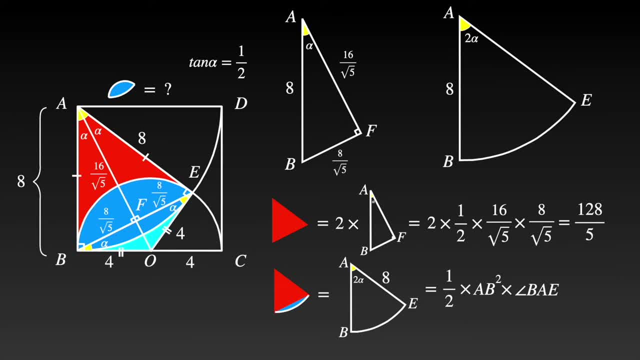 The area of the sector is equal to one half times AB squared times 2 alpha And substitute AB and alpha in We got the result is equal to 64 times arc tangent of one half. Put them aside And consider the right triangle, OBF. 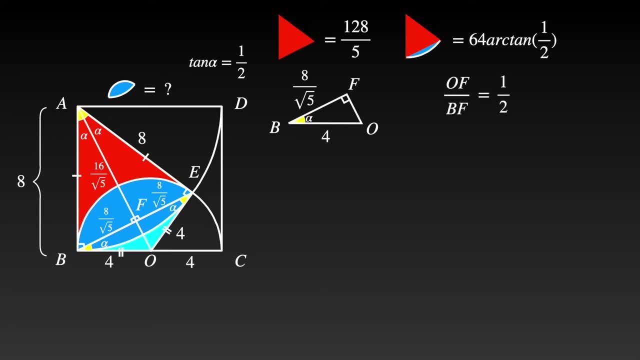 OF over BF is equal to tangent alpha, which is equal to one half, And BF is equal to 8 over square root of 5, as we just solved out, So we can get OF is equal to 4 over square root of 5.. 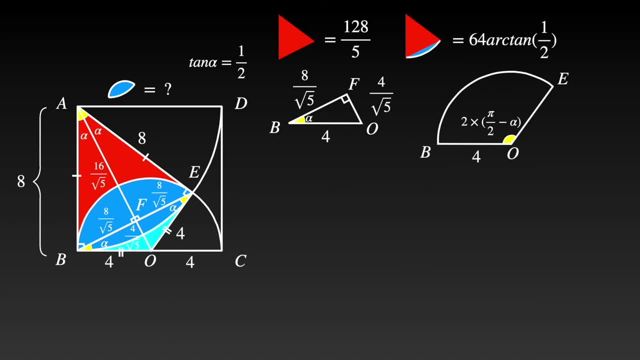 In the sector OBE. OB is equal to 4, as mentioned above, and angle BOE is equal to 2 times pi over 2 minus alpha. So the area of the green triangle is equal to 2 times the area of the right triangle, BOF. 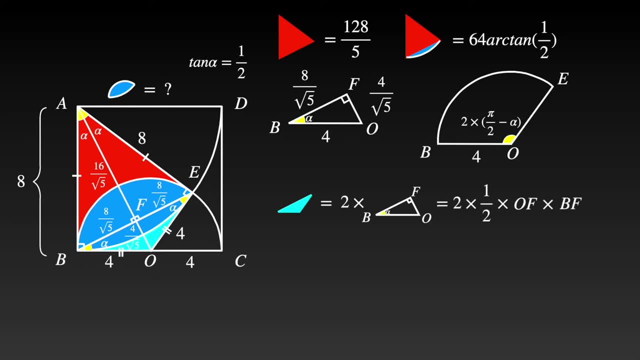 Which is equal to 2 times one half times OF times BF. Substitute the side lengths of OF and BF, We got the result is equal to 32 over 5.. The area of the sector is equal to one half times OB squared times angle BOE.